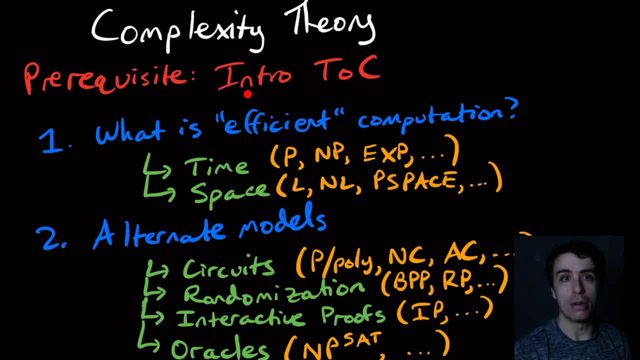 here is that you have to know the things from the intro theory of computation stuff. So there's a playlist that's in the video description. If you haven't watched that, I would suggest that you do so, because you will need it to be able to understand these. So the main questions that 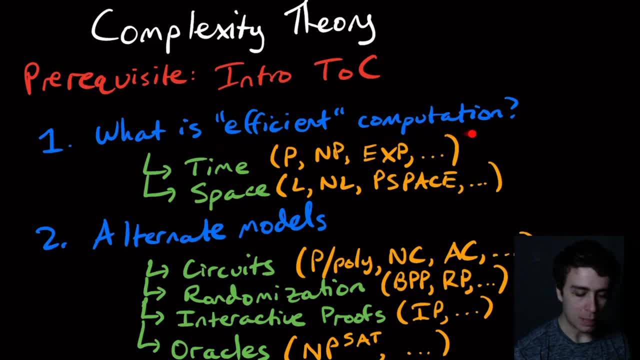 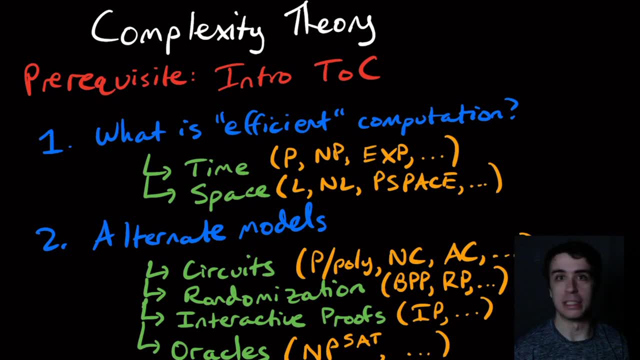 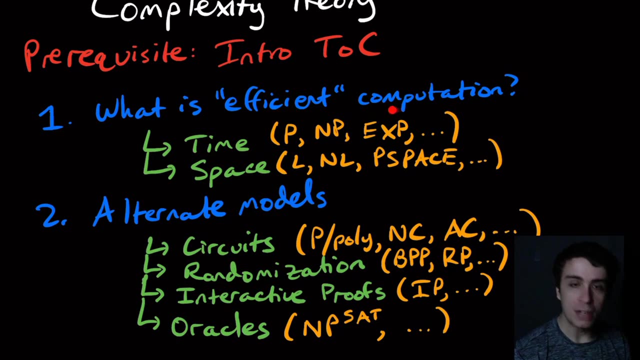 we're going to answer here are: what does efficient computation mean? and some alternate models, at least in this first complexity theory series. There are probably going to be more than this, So the questions that we're going to ask here are: what does efficient computation mean? 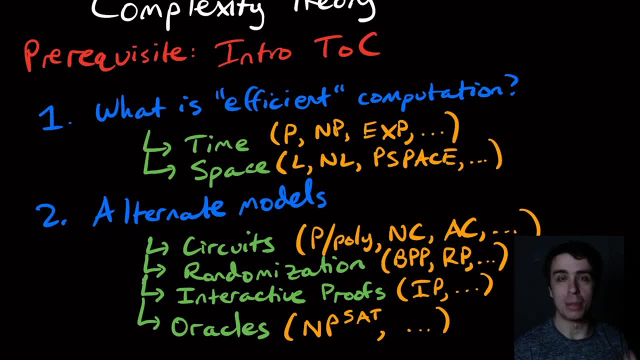 Well, in the intro series we talked about decidable and undecidable languages. Here we are focused entirely on decidable languages, no undecidability stuff. So among the problems that we can solve, how fast can we solve them or how efficiently can we solve them? 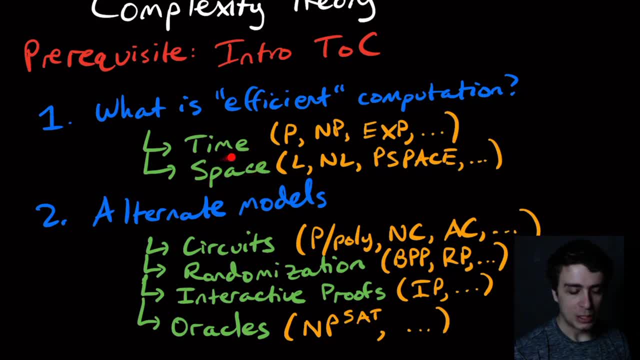 So some of the factors that you may want to consider are how much time something takes or how much space something makes. So if I'm reading a bunch of Twitter tweets that are going right by me, I can't store all of them, So I need to maybe solve a particular problem, maybe classification. 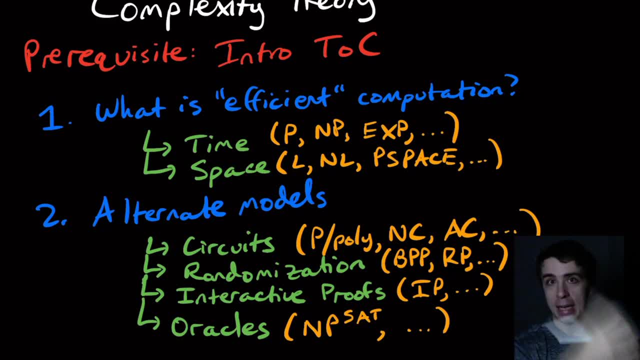 in a very small amount of space, And I don't really care about time. I really can't afford too much space. So space used to be a big deal when you're dealing with relatively small problems, and time used to also be a big deal. But the thing is that computers are so fast now that we start to 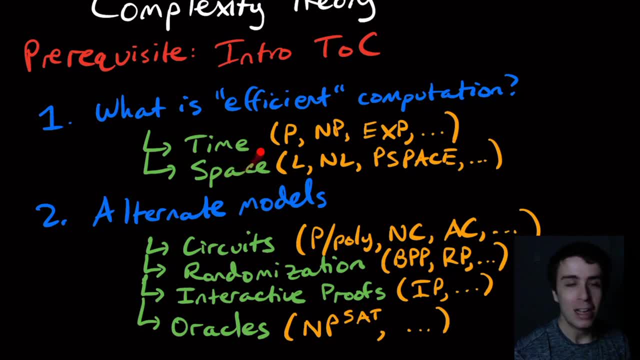 have to process more time. We're actually going to be talking about many of those later, So first I'm going to talk about my Lemma certificate. Um, I didn't really have a lot of time to discuss about this, although for big data. 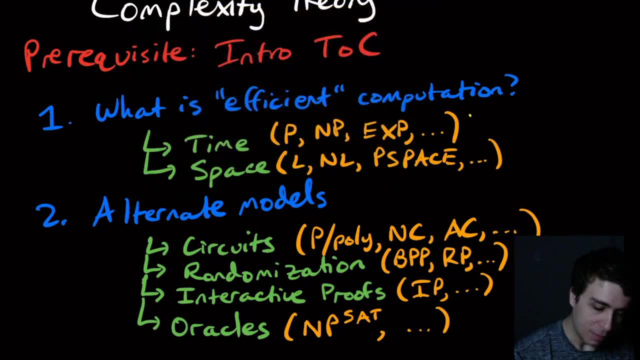 you kind of worry about both of these, but here are some of the topics that we'll be talking about. So P, NP and EXP here they correspond to classes that i want to recognize- how fast can i do it? and there are certain classes that will correspond to. 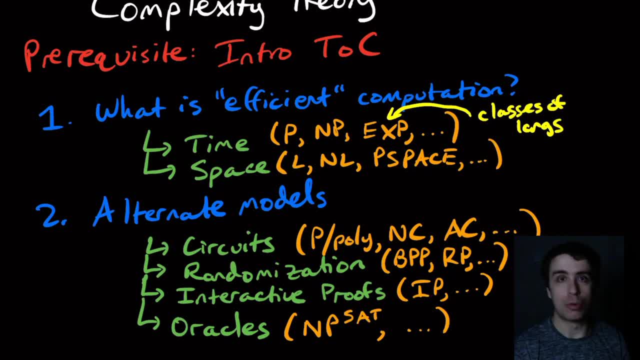 something that's being efficient or not efficient or has some property that we want to satisfy. so p corresponds to, for example, uh- deterministic polynomial time, and np is non-deterministic polynomial. exp, as you might expect, is exponential time and the main question that we ask in 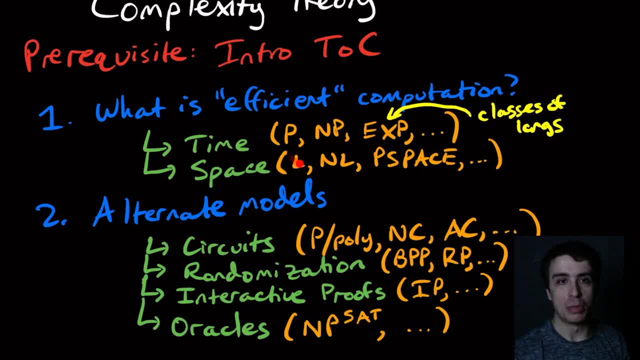 complexity theory is: how did these classes relate to each other? so, uh, how does p relate to np? how does np relate to x? how does any one of these three relate to the space ones? how do any of these relate to any of these down here? so we try to classify sets of these languages in terms of: 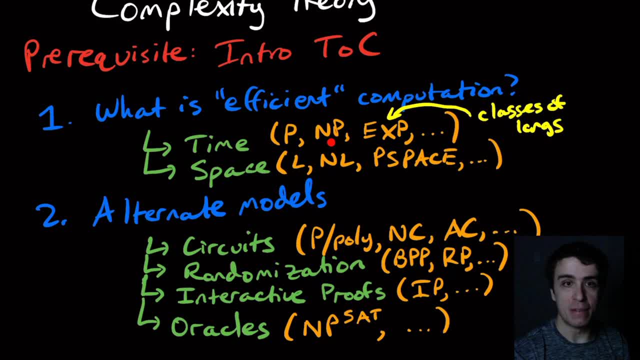 the other ones. so like, for example, p is a subset of np, which is a subset of x, and the only thing that we know is that p is not equal to x. we don't know whether np is not equal to x or p is not equal to np. there's a lot of open questions here and we're not going to be able. 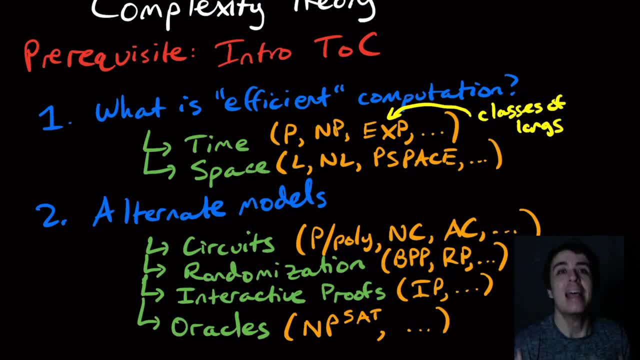 to solve all of them but or really any of them. but it's just mainly trying to see what the connections are between these classes. but another one you may think about is like how much space something use, i don't care how long it takes, i just care about how much space i use. 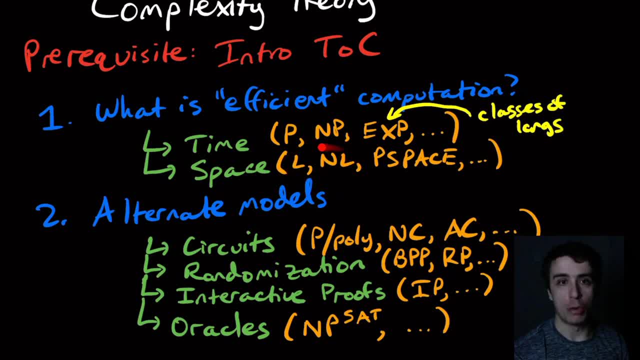 and these classes down here represent log space and that you may think. well, the input is linear. how do you work with logarithmic space? well, we'll see. P space corresponds to polynomial space, as you might expect, and, as an example, NP is a subset of P space, which is a subset of 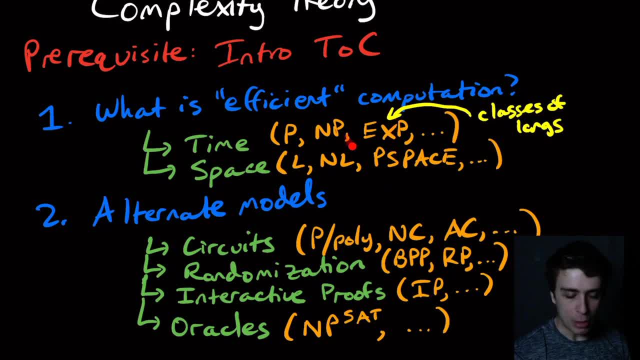 X, but we don't know whether any of these are different from each other, and there's a whole lot of other questions that we need to ask about here. but there are other time classes and space classes that you may want to consider also. it's not just these, but these are the ones we're going to at least talk about here. 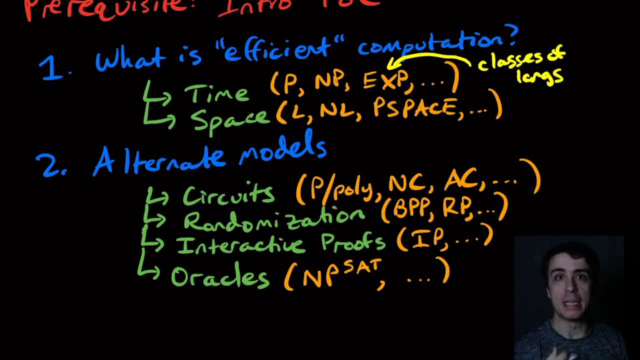 but there are other alternate models of computation so these ones are based on a Turing machine running on some input. some other models you may want to consider: our circuits. so a lot of electrical engineers like to build circuits that solve a particular problem. and how efficiently can we solve? 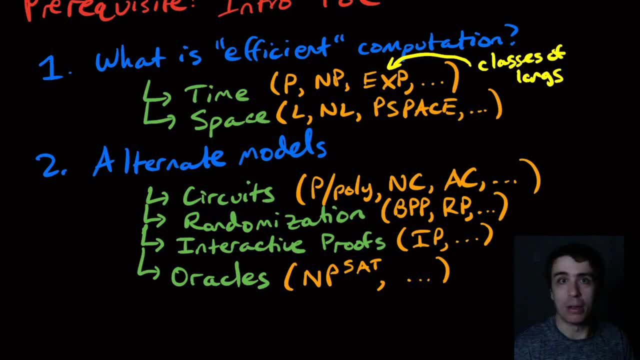 problems using circuits and it's not quite the same model and so we can ask different questions and get slightly different answers. so P, poly is a class and it may. it seems kind of weird what it means, but we're gonna talk about eventually- and C cores and AC correspond to the limiting the circuit in some way. so you can't. 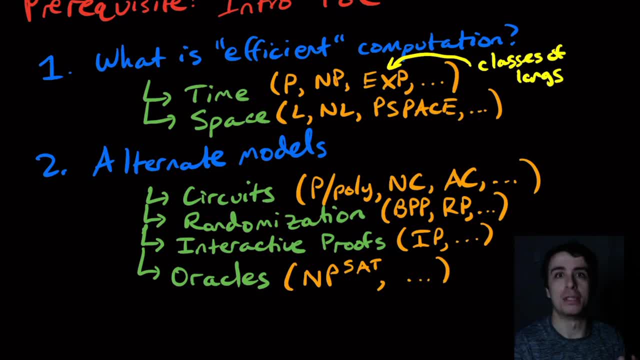 have any arbitrary circuit, but we can have certain types of circuits, and NC stands for Nix classes, for example, and that corresponds to: well, how efficiently can I parallelize something? so one example is that we, you can show that NC is a subset of P and you may ask the question: well, this class corresponds to the things that are. 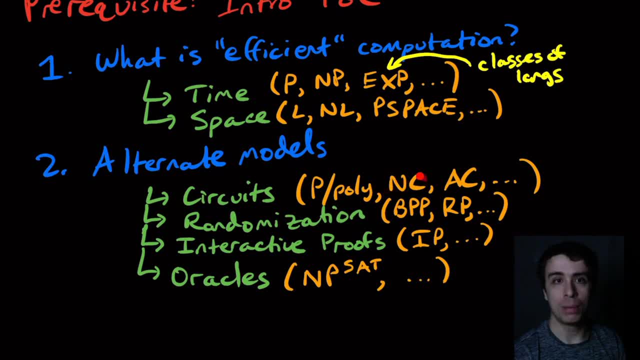 efficiently in some sense parallelizable? and then we don't know whether P is equal to NC. so the question there is: is every problem that's efficiently solvable parallelizable also? and we don't know the answer to that. but another model is randomization, so we may not be able to solve a problem perfectly. 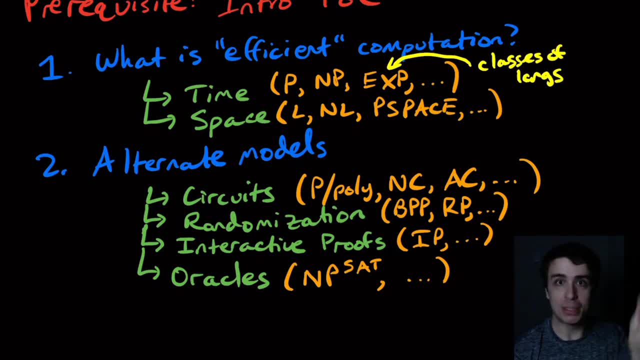 exactly, but maybe we can get a very small epsilon away from the true answer. we may answer wrong some of the time, or maybe we don't get the optimum answer, but we can get pretty close and we ask- well, if I need just allow a little bit of error- how? 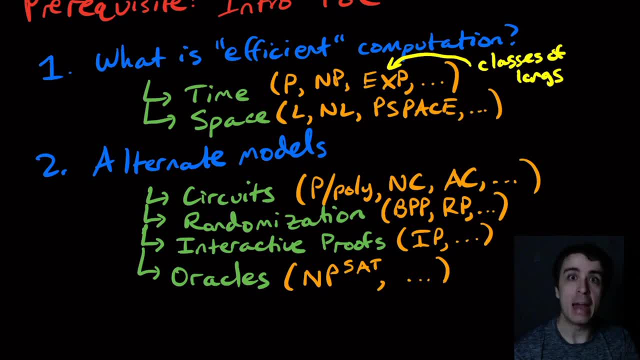 how efficiently can I solve problems within the error tolerance? and these classes that we'll talk about here are trying to see, if I allow for randomization, how much different are they from these? so if you have some error, then clearly you can do at least as well as you did in the deterministic. 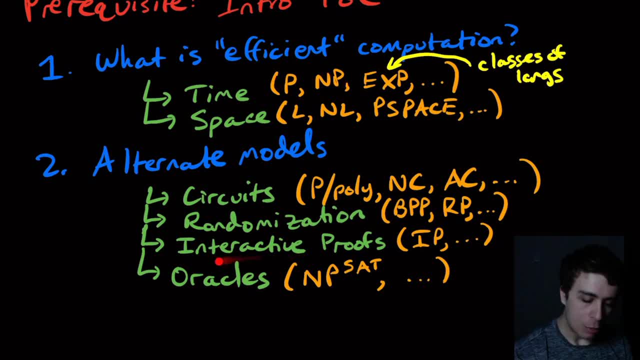 setting, but it's just how much better interactive proofs. so if you this is entirely different model and you're just trying to do a randomization where you don't have any error in the first place, then there's not a possibility of having any error in the second place, only if your test system 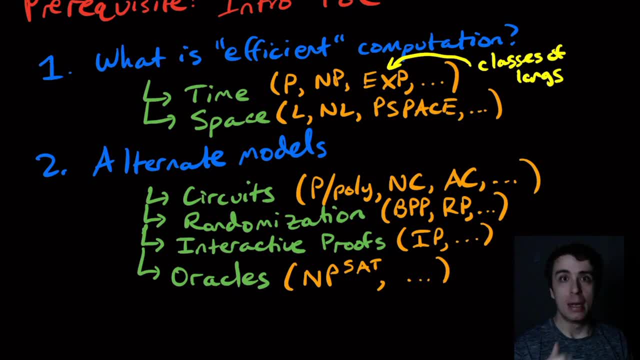 is all the way through and you get an error for this and you can into an automated test. so this is a very common procedure. so if you have a test, that's what the prover is saying and there's a back and forth, that happens and you can talk about. 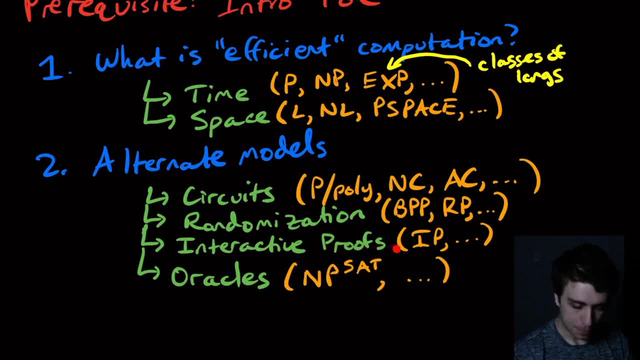 certain problems that are recognized in this setting, And one thing that we'll show is that IP, which is the set of languages that are solvable using this interactive proof setting, in some sense is equal to PSPACE. So that's one amazing result that we're able to prove. 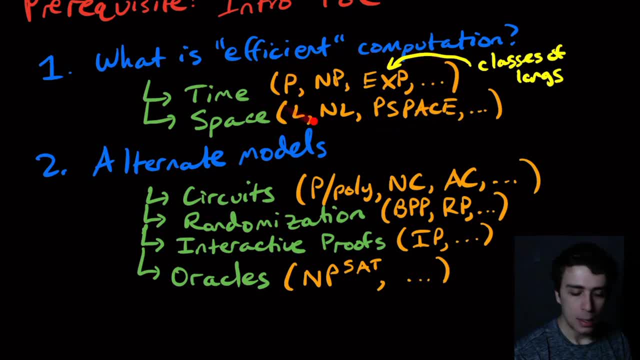 Um, and also for here. all of these, in fact all of these really have complement versions which we have some open questions about and some that we don't we can actually solve. So like, for example, NL is closed under complement, P is closed under complement, I think XSP is, PSPACE is, but 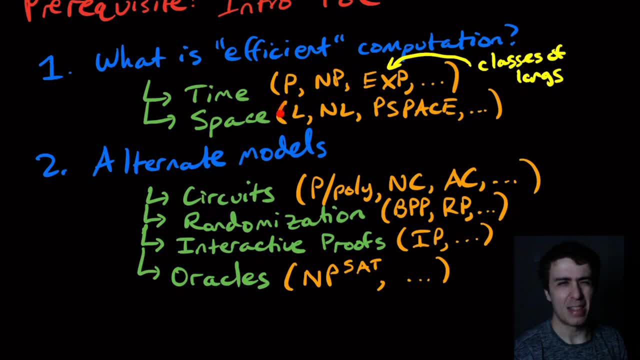 we don't know whether NP is closed under complement. I think L is, I'm not sure. I have to think, Uh, but NP, NP is not, is not known to be closed under complement, for example. So there are a lot of. 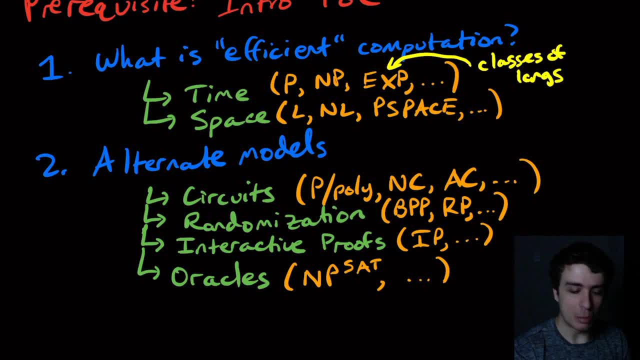 properties that we've talked about with, say, DFAs that we can apply here, and there are a lot of open questions there. Another one is oracles. So an oracle is basically, if I can immediately solve a particular problem, uh, in zero time, assuming that we can then allowing ourselves non-deterministic. 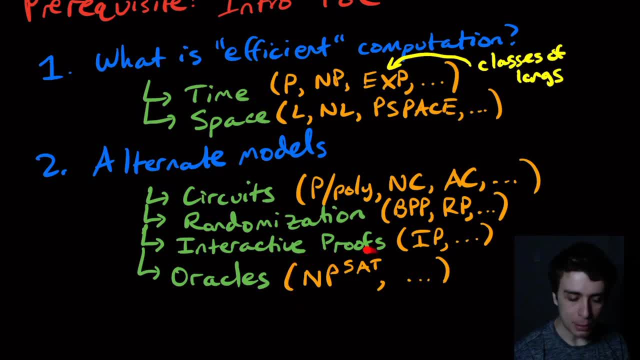 polynomial time, in addition, to be able to solve this problem, uh, instantaneously. what kinds of problems can we solve then? The one of the only reasons that we consider oracles is that we want to separate, show some kind of separation, or at least some kind of evidence toward a separation. So, for example, 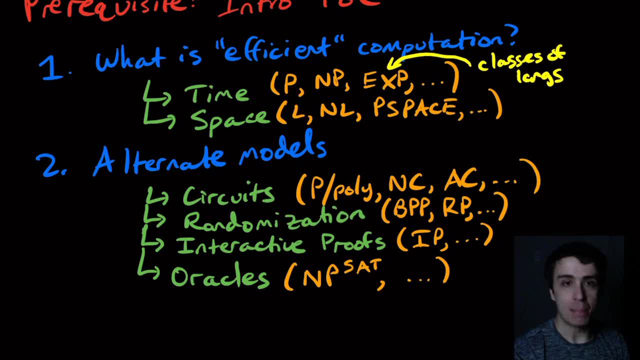 um, we don't know whether P is equal to NP, but if I provide you any uh instantaneous access to some uh language, can I separate the two in that setting? And if you can, then that would give you some evidence that they are uh in fact different. It doesn't give a proof, but it gives.